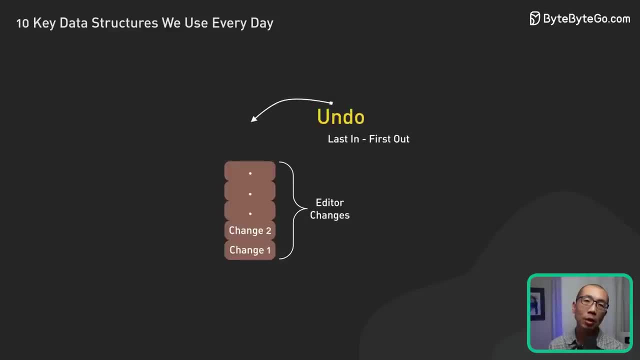 making it simple to revert to a previous state when the user triggers an undo operation. Next, we have stacks. Stacks can be used to store each change made to the text, making it simple to revert to a previous state when the user triggers an undo operation. 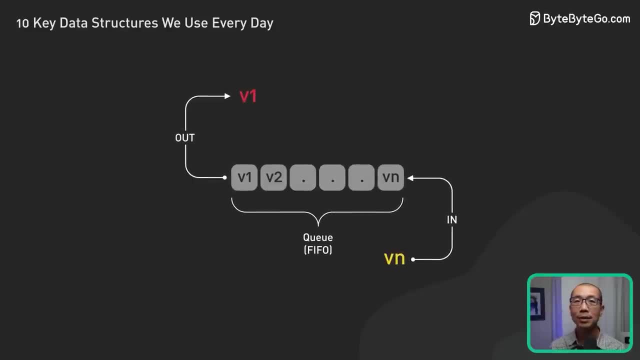 Next we have stacks. Stacks can be used to store each change made to the text, making it simple to revert to a previous state when the user triggers an undo operation. Kiosk operate on a first-in, first-out basis. They are good for managing printer jobs. 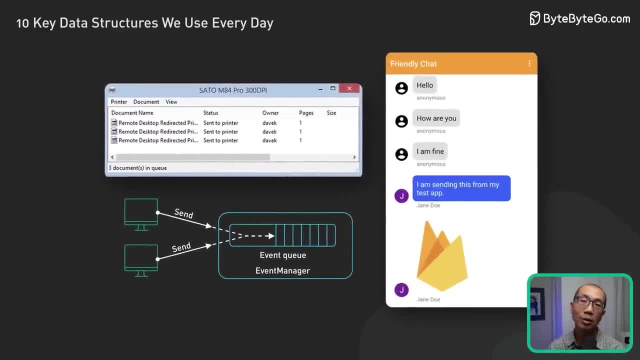 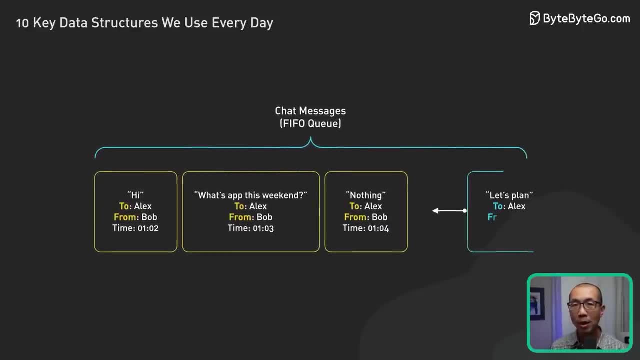 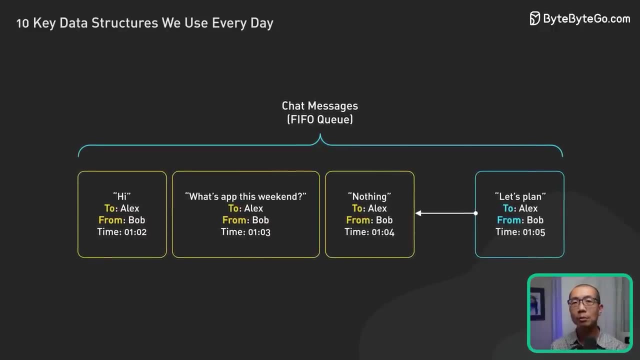 sending user actions in games or handling messages in chat applications. In chat applications, a kiosk can be used to store incoming messages in the order they are received. It ensures that they are displayed to the recipient in the correct sequence. Heaps, on the other hand, are used for tagging. 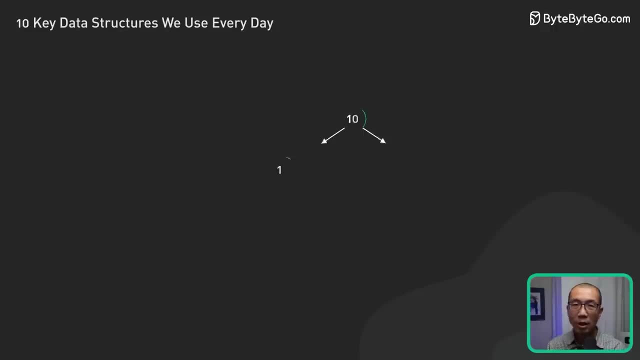 They are especially helpful in implementing priority queues, where we need to access the highest or lowest priority item efficiently. Trees organize data hierarchically. They are useful for representing data with natural hierarchies or relationships. They can be used in various applications like database indexing, AI, decision-making or file systems. 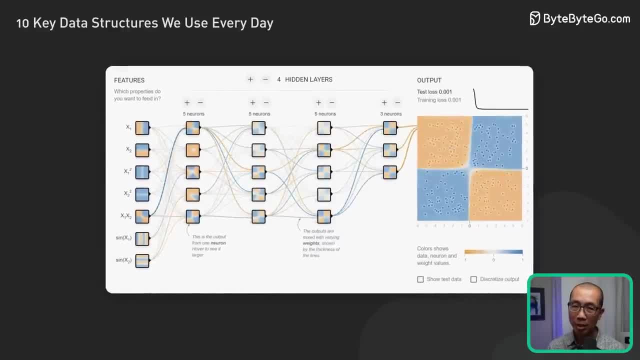 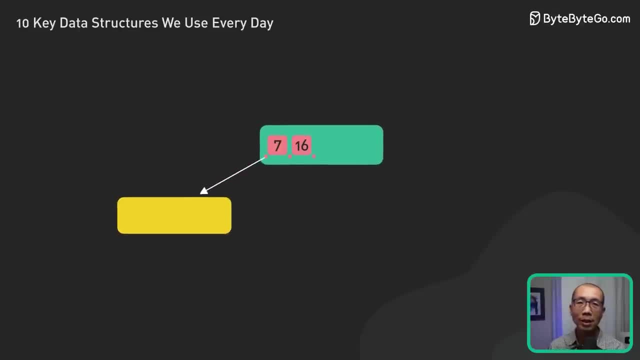 In AI. decision-making trees, like decision trees, are used in machine learning for classification tasks. Trees are also used in database indexing, where they can help speed up search, insert or delete operations. For example, B-trees and B-plus-trees are commonly used in relational databases to efficiently manage and index large amounts of data. 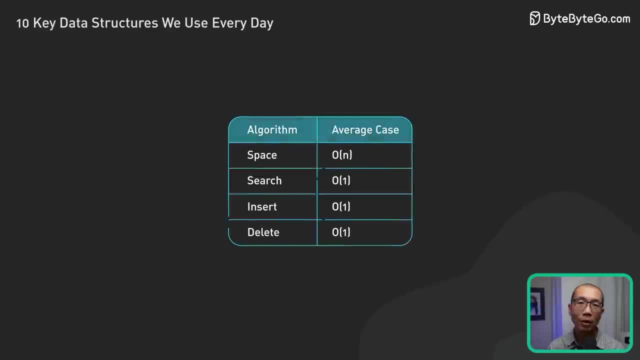 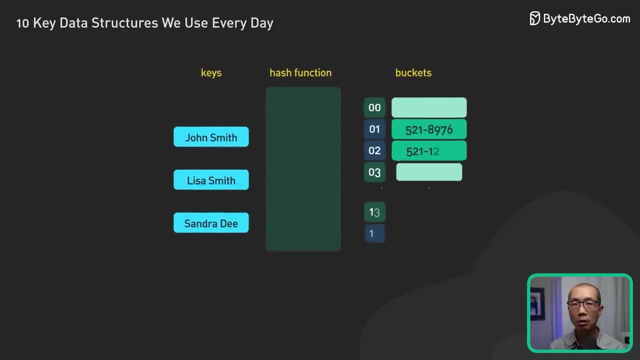 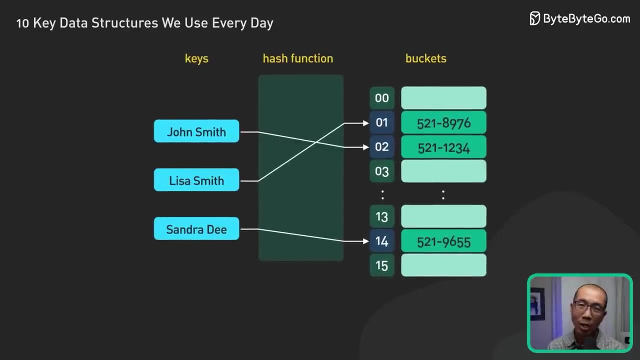 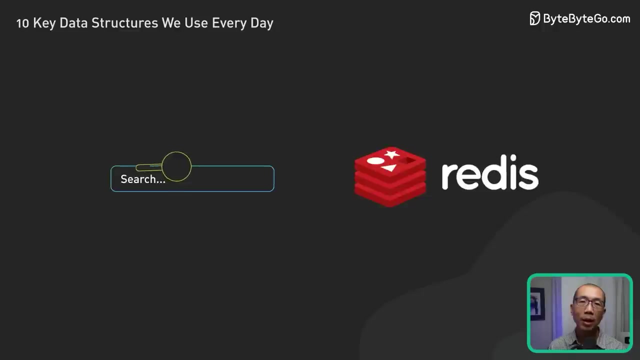 Hash tables allow for efficient data lookup, insertion and deletion. They use a hash function to map keys to their corresponding storage locations. It enables constant-time access to the store values. Hash tables are widely used in various applications such as search engines, caching systems and programming language interpreters or compilers. 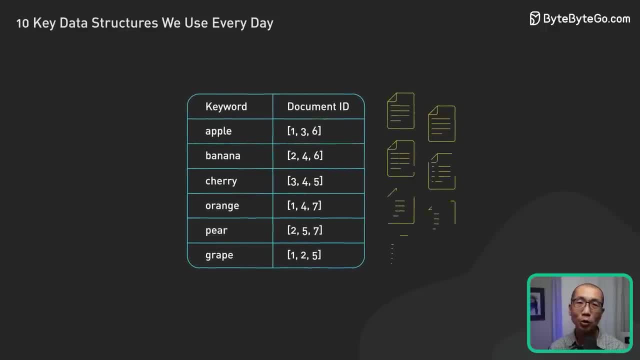 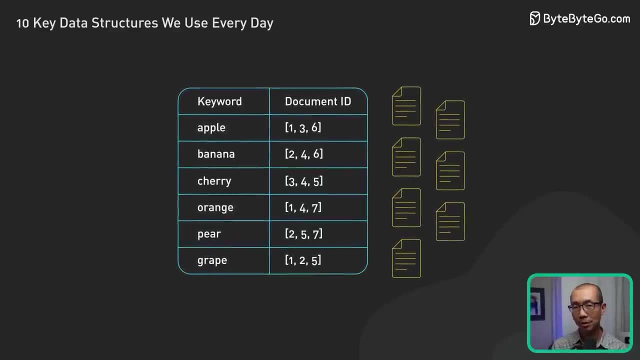 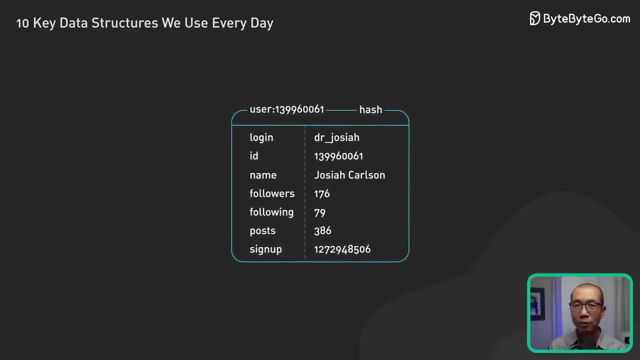 In search engines. hash tables can be used to store and quickly retrieve indexed data based on keywords. This provides fast and relevant search results. Caching systems may use hash tables to store and manage cached data. It allows for rapid access to frequently requested resources and improves overall system performance. 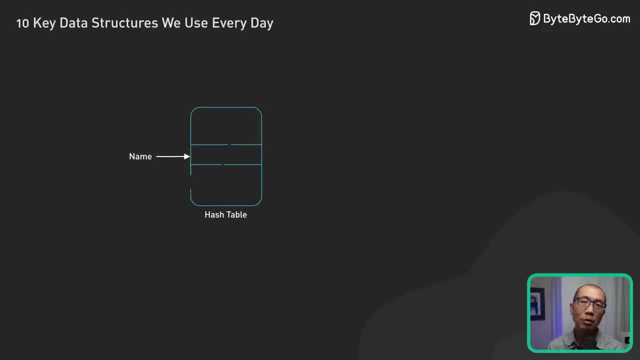 Another example is the implementation of symbol tables in programming language interpreters or compilers. Hash tables can be used to efficiently manage and look up variables, functions and other symbols defined in the source code. Suffix trees are specialized for searching strings in documents. 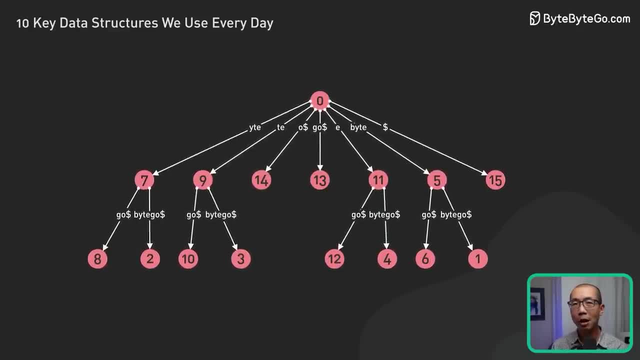 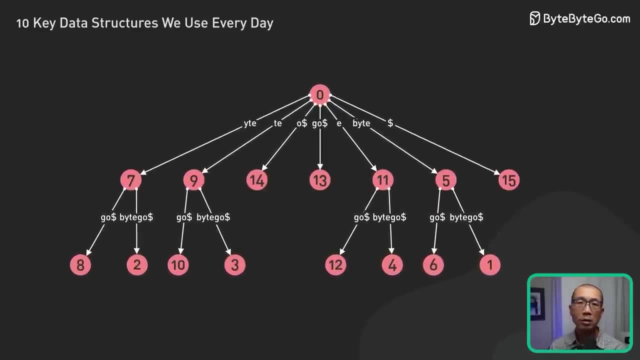 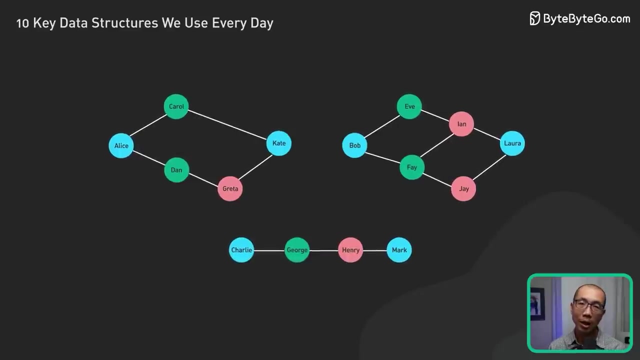 This makes them perfect for text editors and search algorithms. In a search engine, a suffix tree can be used to efficiently locate all occurrences of a search term within a large corpus of text. Graphs are all about tracking relationships and finding paths. This makes them invaluable in social networks, recommendation engines and path-finding algorithms. 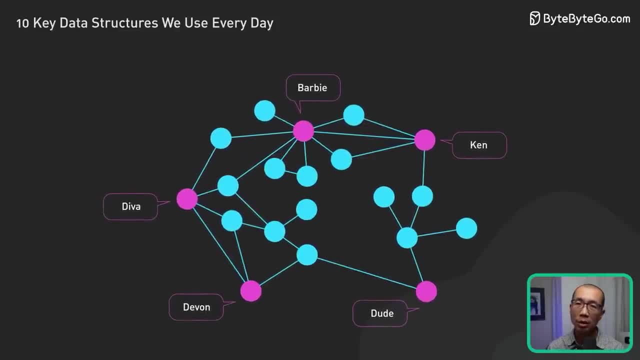 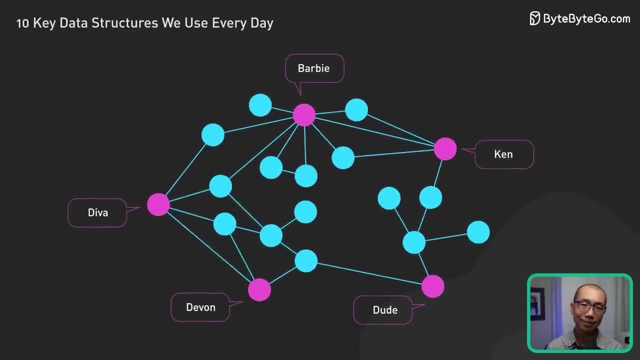 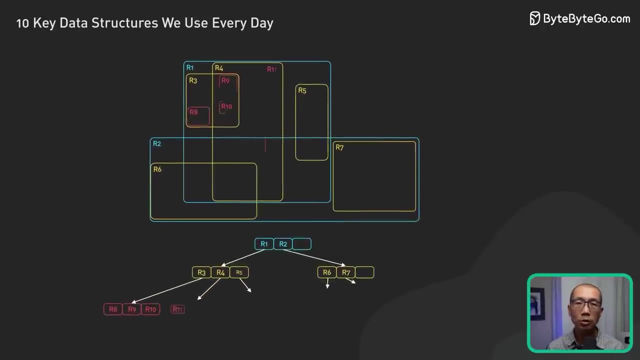 In a social network. a graph can be used to represent the connections between users. It enables features like friend suggestions or analyzing network trends. R-trees are good at finding nearest neighbors. They are crucial for managing the search results. They are crucial for mapping apps and geolocation services. 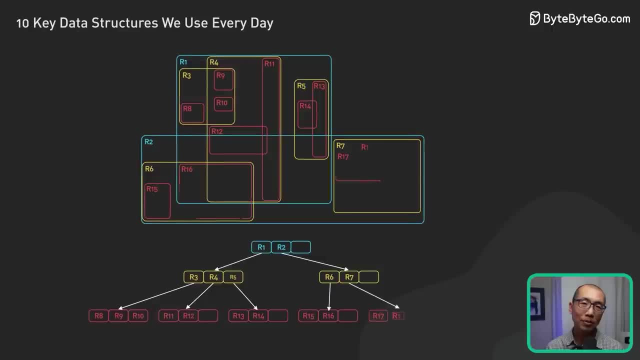 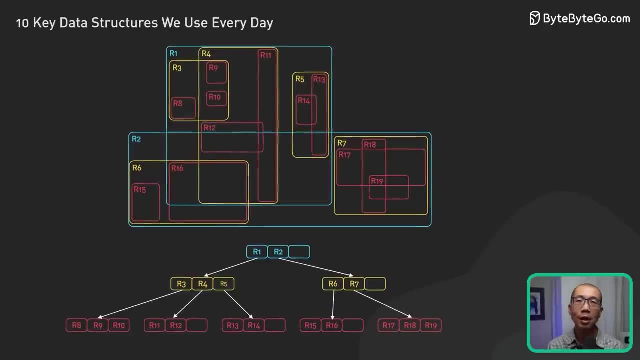 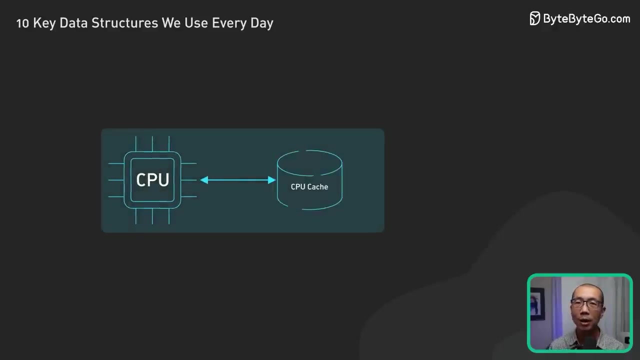 In a mapping application. R-trees can be used to store spatial data such as points of interest. This enables efficient queries to find the nearest locations based on the user's current positions. Now let's discuss cache friendliness and how it relates to various data structures. 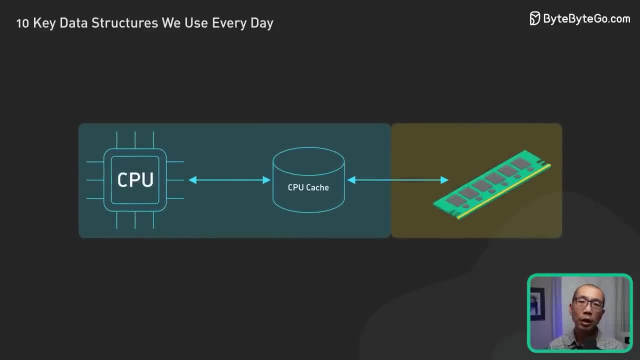 including lists, arrays and other mentioned earlier in the video. CPU cache is a small fast memory between the main memory and the CPU. It stores recently accessed data and instructions so the CPU can access them quickly without fetching them from the slower main memory. 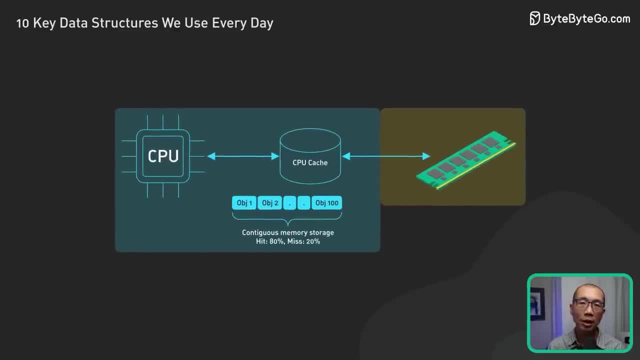 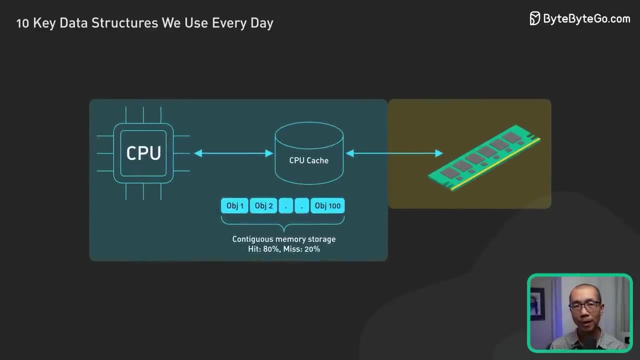 Different data structures have varying levels of cache friendliness based on how their elements are stored in memory. Contiguous memory storage, like that in arrays, allows for better cache location. This allows for more cache mentality and fewer cache misses, resulting in improved performance. 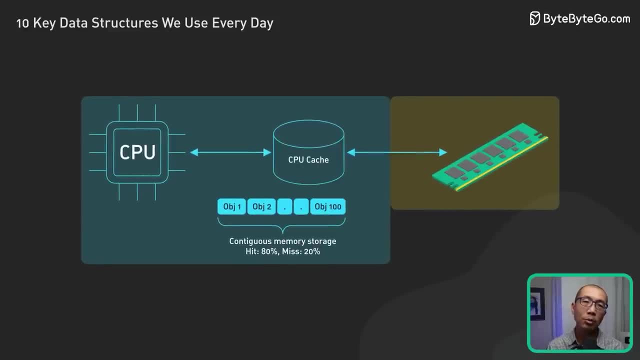 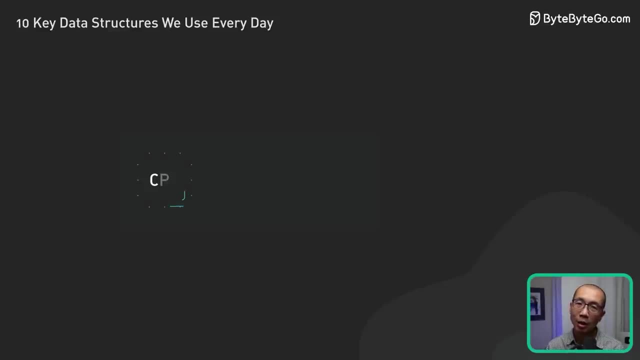 When an array element is accessed, the cache can prefetch and store nearby elements, anticipating that they might be accessed soon. On the other hand, data structures with non-contiguous memory storage, like linked lists, can experience more cache misses and reduce performance.